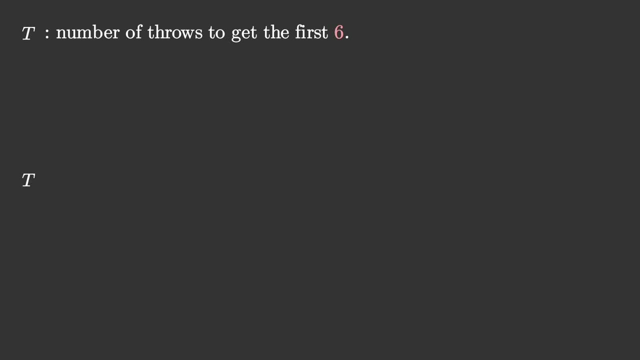 first six And note that t is a random variable, so it would vary from one game to another, And what we're interested in is the expectation of t. So before we derive this expectation, let's actually compute the distribution of the random variable t. So t takes positive integer values only. 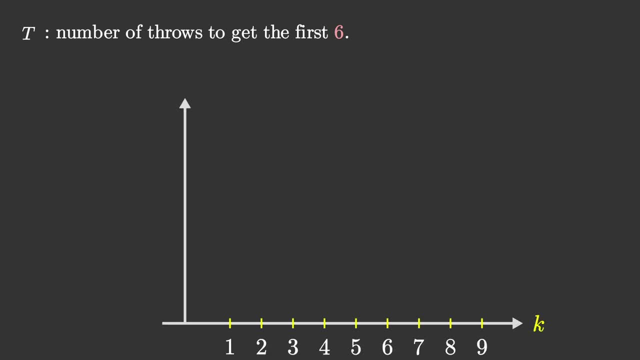 So let's compute the probability that t equals k. for every positive integer k, The probability of t equals one is one over six, assuming the dice is fair. This is because there are two possible outcomes and they are all equally likely. Easy enough. 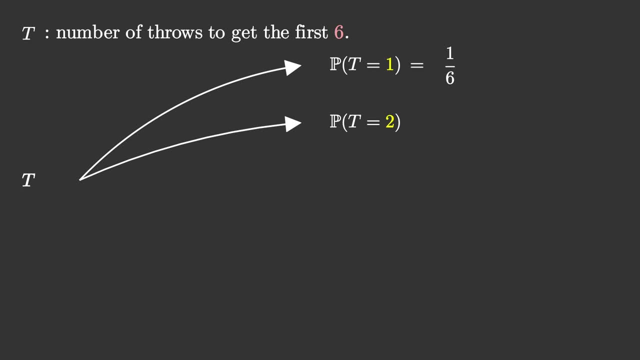 What is the probability that t equals two? Well, we need the first throw to be anything but a six, which happens with probability five over six, and the second throw to be a six, which happens with probability one over six. How about the probability that t equals three? Now, we need the first throw. 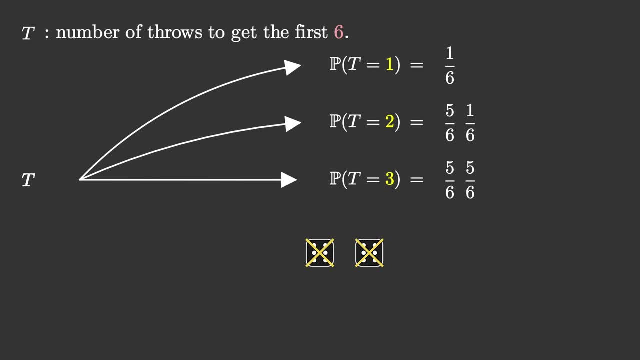 not to be a six, the second throw not to be a six and the third one to be a six. In other words, this probability is given by five over six squared times one over six. More generally, the probability to that t equals k is given by five over six to the k minus one times one over six. 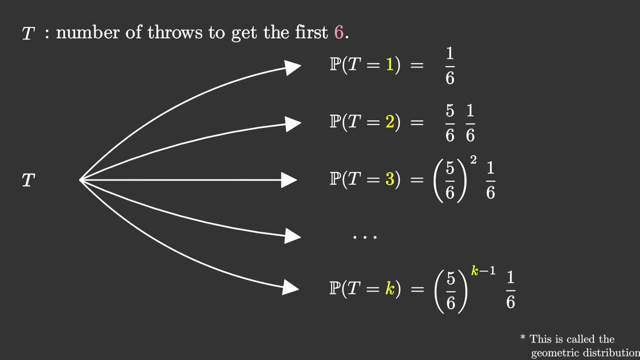 Ok, Cool. Now, in order to compute the expectation of t, what we need to do is multiply each probability with its respective value and take the sum Replacing the probabilities with their corresponding values. our job now is to evaluate an infinite sum. 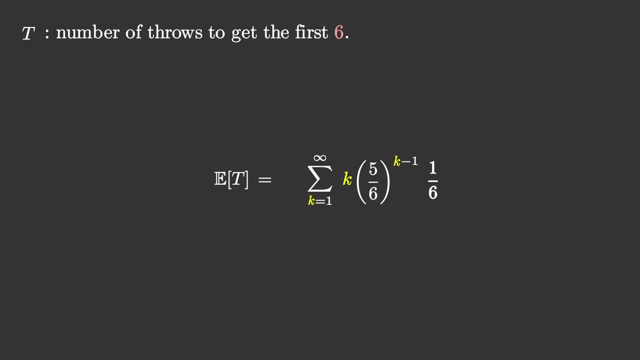 I have warned you that this solution is the most computational, and now we see why. Anyway, we have come this far and we're not going to stop so close to the goal. The first thing I'm going to do now is pull the 1 over 6 out of the sum, since it is a constant. 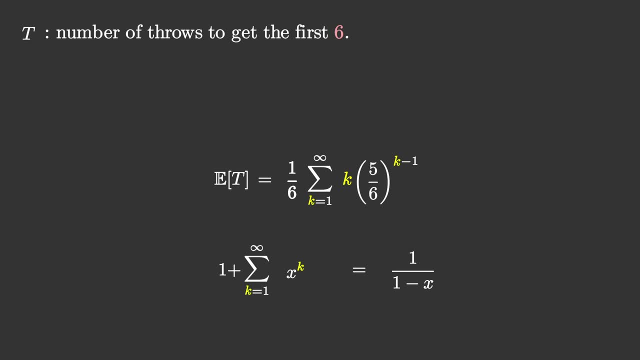 Next, I'm going to use a neat little formula known as the infinite geometric series. We will take derivatives of both sides of this identity. The derivative of the right-hand side is 1 over 1 minus x squared, And we're going to take the derivative of the left-hand side, which is 1 over 1 minus x squared. 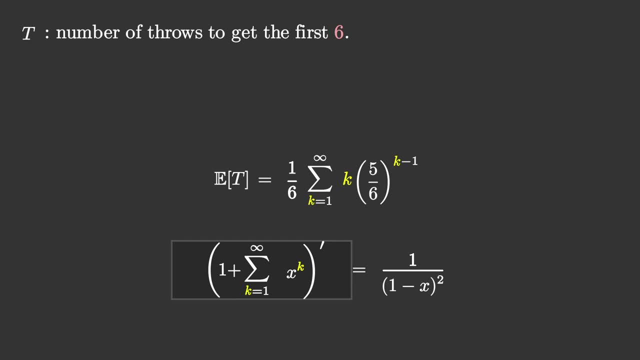 And we're going to take the derivative of the right-hand side, which is 1 over 1 minus x squared, And for the left-hand side, we're going to take the derivative term by term And we're going to use the fact that the derivative of x to the k is given by k: x to the k minus 1.. 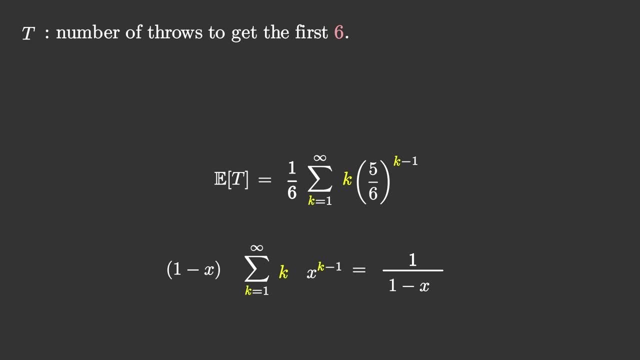 We multiply the left-hand side and right-hand side by 1 minus x, And finally we replace x with 5 over 6.. And lo and behold, the left-hand side is exactly the formula that we found for the expectation of t. 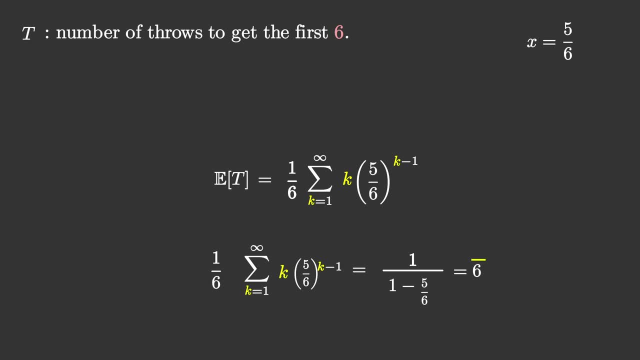 And the right-hand side simply evaluates to 6.. The answer turns out to be surprisingly clean, despite the fact that the formulas we used were kind of messy. You might wonder if there is a better way to go about this problem, And indeed there is one. 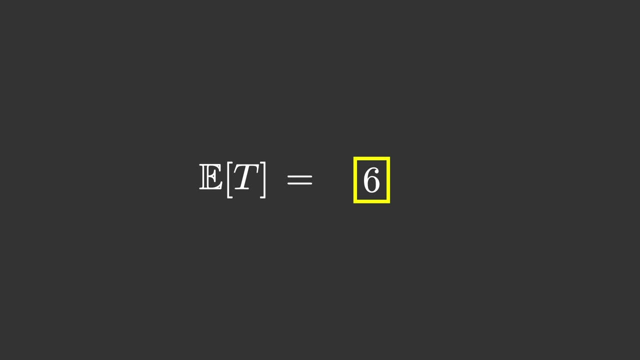 And that's what we will do next. Before we do that, though, we make a few observations. Incidentally, the answer happens to be 6,, which is the face of the data, And that's the dice we were looking for. 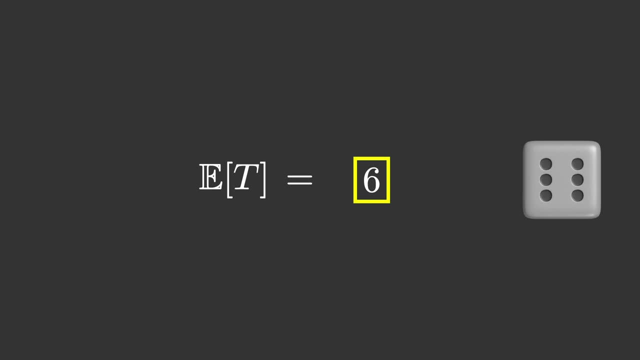 This is easily seen to be just a coincidence, though, since the answer wouldn't change if the game had stopped after, say, a 4 rather than a 6.. The 6 actually comes from the fact that the probability of getting any number from a fair dice is 1 over 6.. 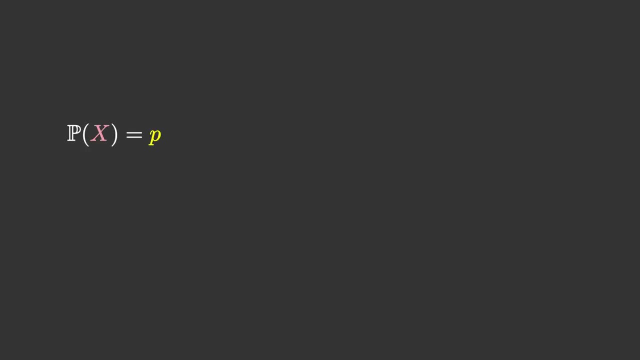 And, more generally, if an event has probability p of happening, we expect that it would take 1 over p tries before the event happens for the first time. For example, it would take 2 coin flips on average to get the first head, since the probability of getting a head or a tail is 1 half. 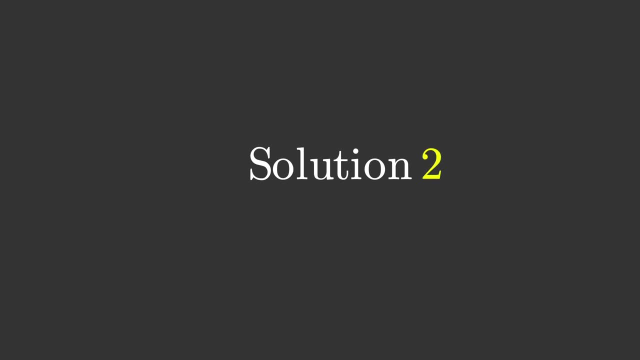 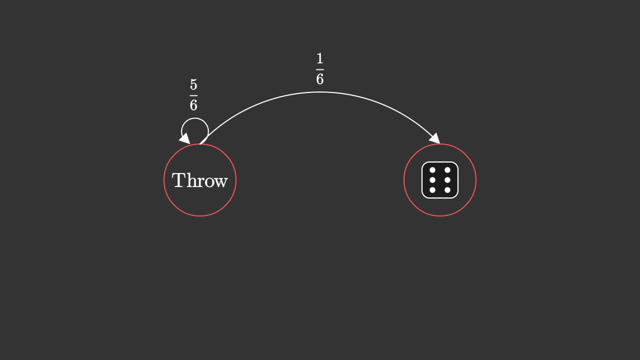 Otherwise you get a 6. With probability 5 over 6, you get some other number and basically you have just wasted a throw and you have to start all over again. Hence the recursion. If we untangle this diagram, we get this repeating or recursive structure. 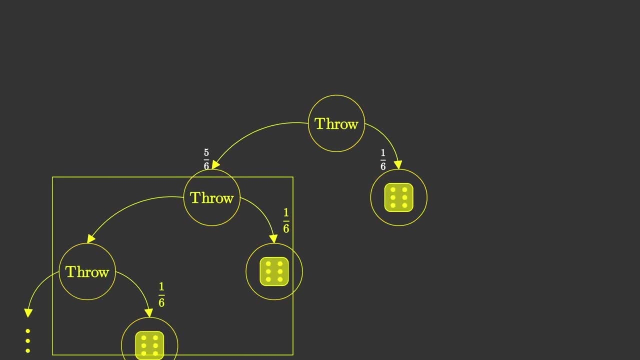 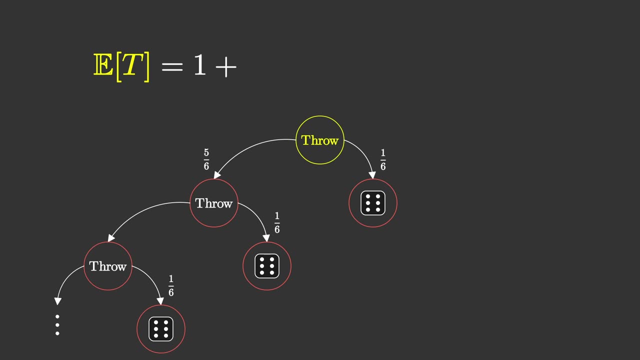 The left child node is always similar to the full tree, And it becomes clear from here that the expected number of throws after the first throw is 1 over 6 times 0, plus 5 over 6 times expectation of t. 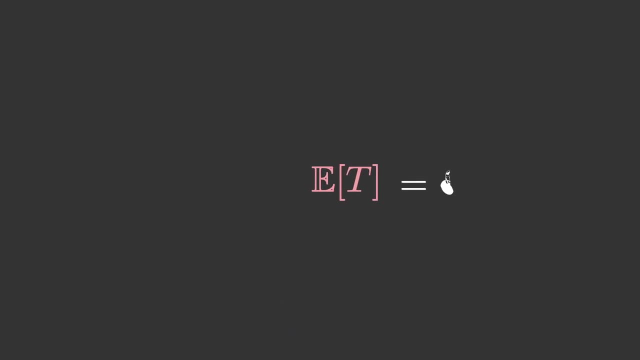 Solving this equation directly leads to expectation of t equals 6, which is nice. An unexpected consequence of this way of solving the problem is that we recover the value of the infinite sum of k times x to the k minus 1 in a completely different way than we did before. 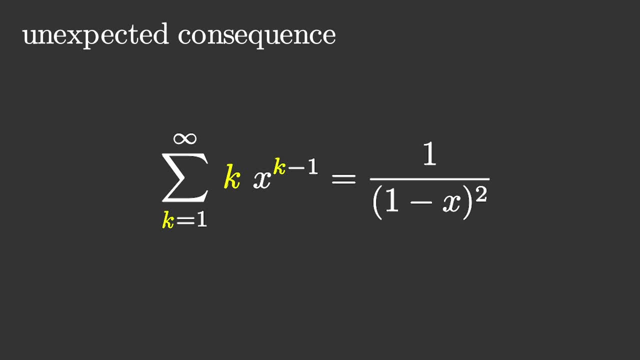 without resorting to a new equation, without resorting to a new equation, to any derivation tricks. For the third and most elegant solution, we will use one of the most profound and yet strikingly simple results in probability theory: the law of large numbers. 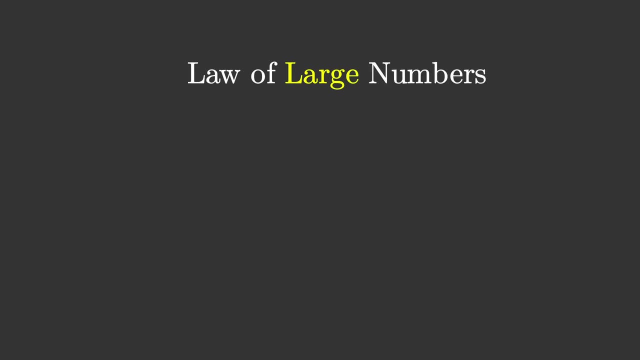 The law of large numbers simply states that as you repeat a random experiment a large number of times, the outcome will converge to the theoretical expected value. For example, if you flip a coin once, you can get either a head or a tail, and it would 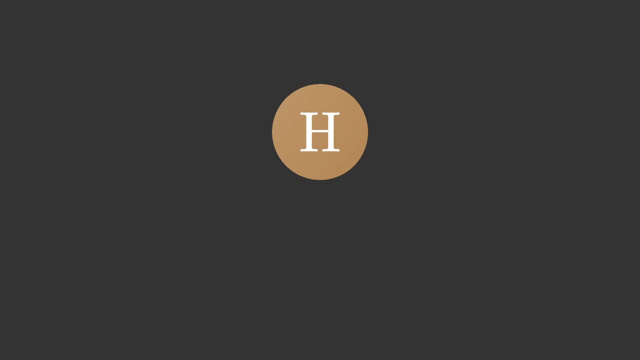 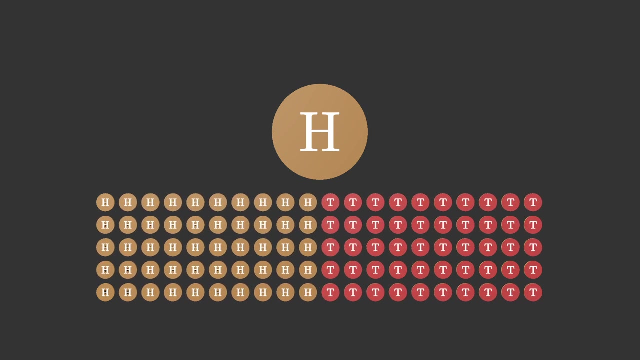 be impossible to tell which one you would get in advance, But if you flip a hundred coins you can predict with some confidence that about half of the flips would be heads and the other half would be tails, and your confidence would grow as the number of flips increases. 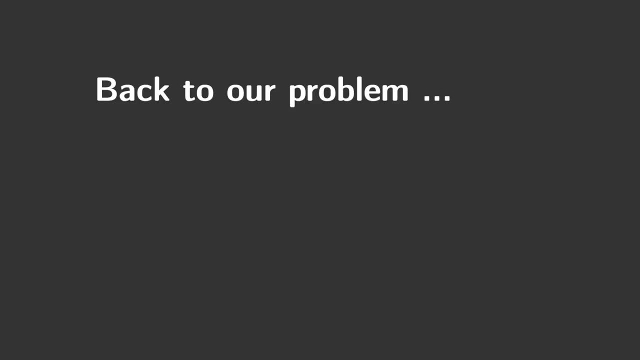 Back to the problem. We will now think a little differently than we did before For the other two solutions. In fact, we will imagine a scenario where you don't play a single game, but a large number of games. I said a large number of games. 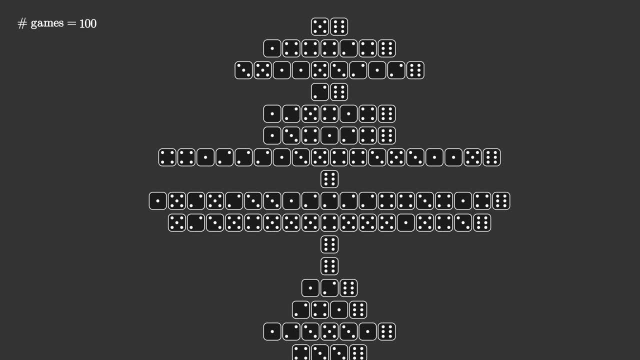 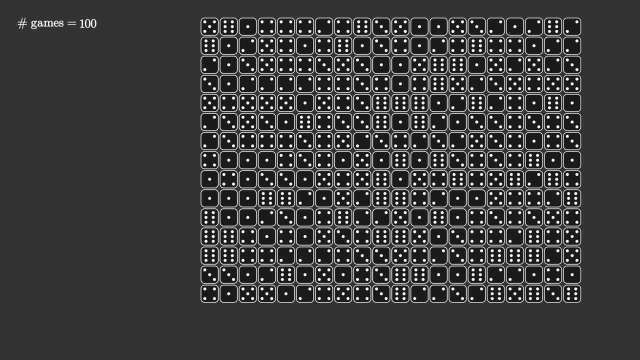 Much better, And we will see in a second why that's useful. And let's put all the throws next to each other so that we have a long sequence of throws. Now notice that every game has to end with a six, So the total number of throws is six. 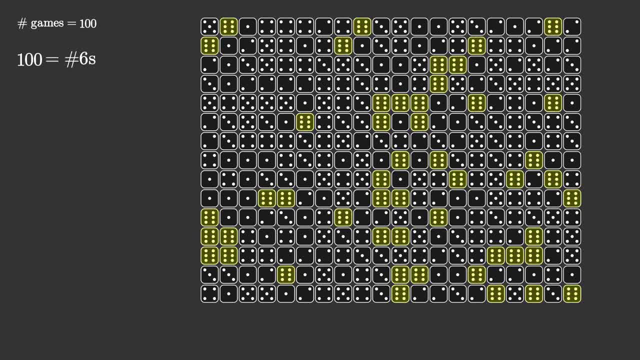 So the total number of throws is six. So the total number of throws is six. So the total number of games is equal to the number of sixes. How many sixes are there in this sequence? We can use the law of large numbers to estimate the number of sixes to be one sixth of the. 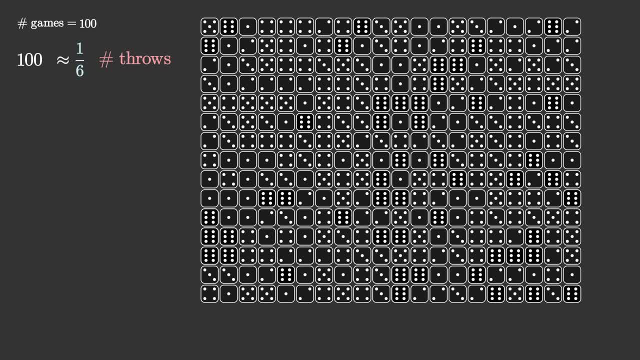 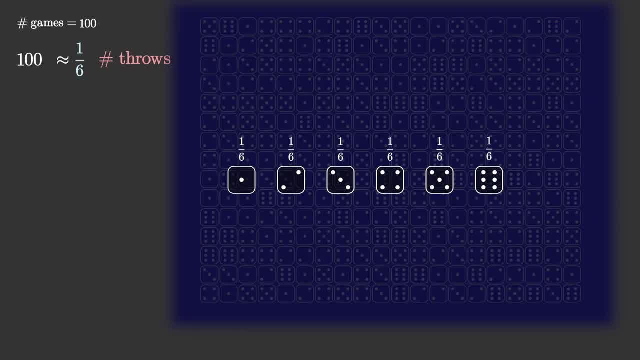 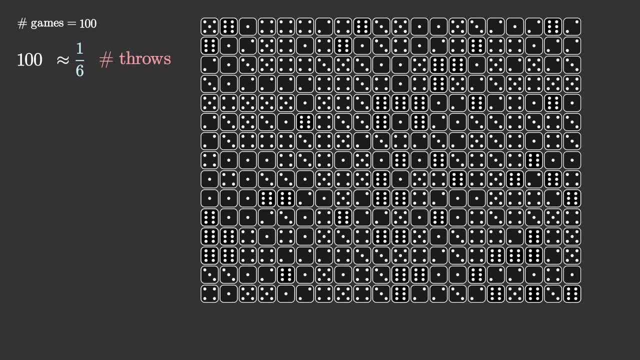 total number of throws. We can also appeal to a simple symmetry argument, since throwing a dice leads to six possible outcomes that are equally likely. So we expect each one of them to appear one sixth of the time, And the total number of throws itself, if we play 100 games, is gonna be 100 times the. 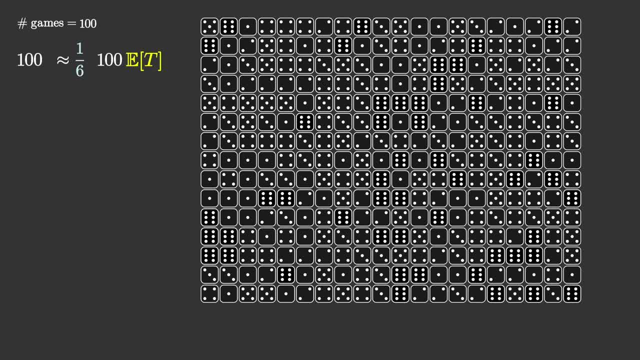 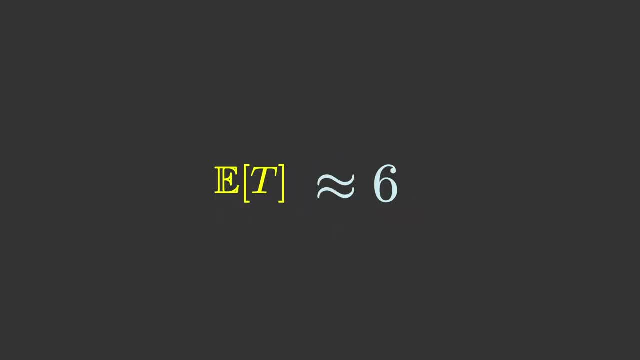 expected length of a single game. After simplification we now have the expectation of t is approximated by six. Note that up to this point we only have an approximation and not an equality. But this approximation gets better and better as the number of games increases and in fact, 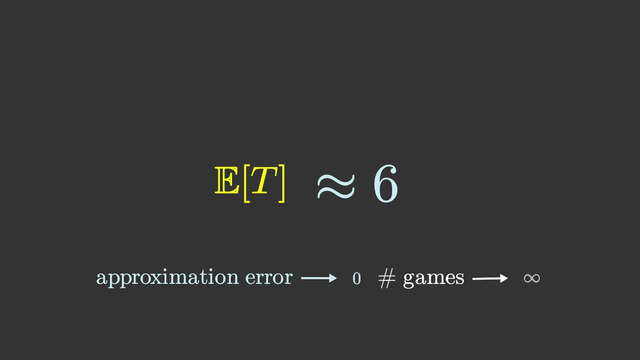 becomes exact, as this number goes to infinity, But since the approximation itself does not depend on the number of throws, then we actually have an equality here. This is one of those times where it feels like we are strengthening a result for free, meaning we go from an approximation to an equality without any extra effort, and this 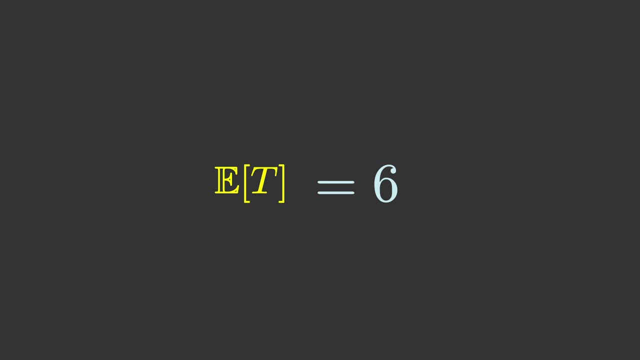 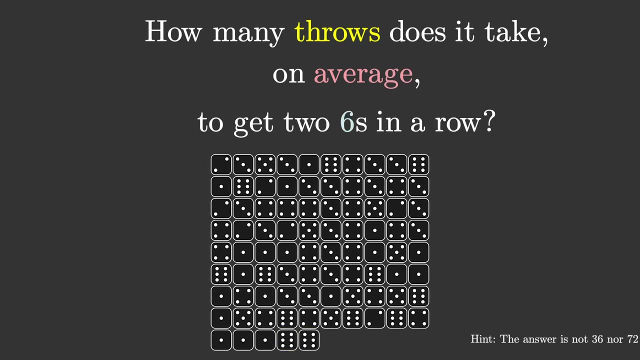 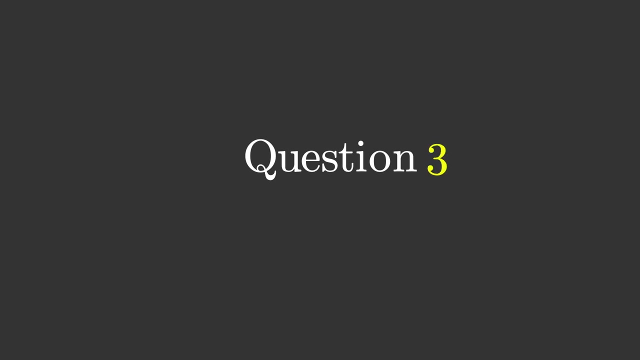 is thanks to the law of large numbers. If you want to check your understanding of the three solutions presented here, try to answer the following questions: • What is the median number of throws required to get the first six? • How many throws does it take not to get one six, but two sixes in a row? 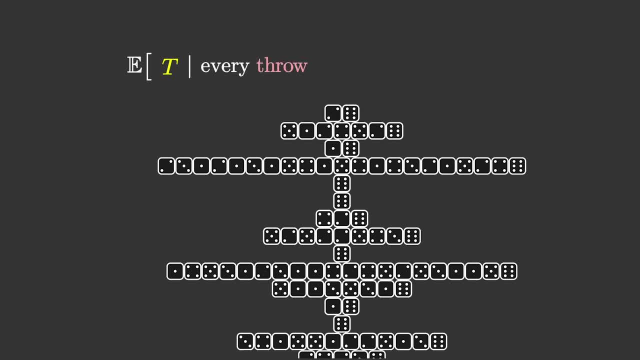 • How many throws does it take to break a spin tackle take to get a 6, conditioned on the fact that all the throws so far were even?